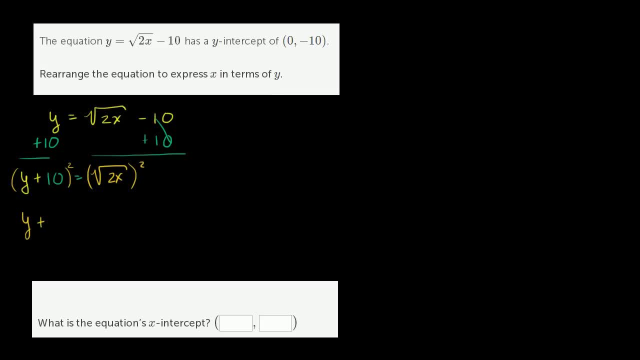 And we are going to have y plus 10.. y plus 10 squared is equal to the square root of 2x. squared is just going to be 2x is equal to 2x, And now we can divide both sides by 2.. 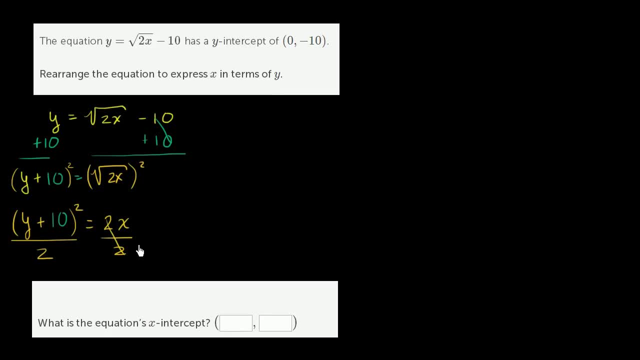 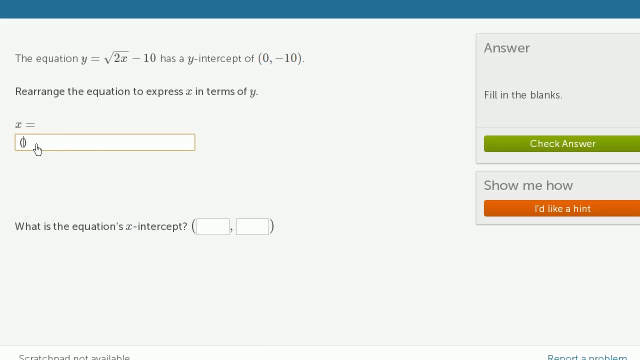 Divide both sides by 2.. And we are left with x is equal to y plus 10 squared over 2.. So let me write that out, Let me actually type that into the program right over here. So x was equal to y plus 10 squared over 2,. 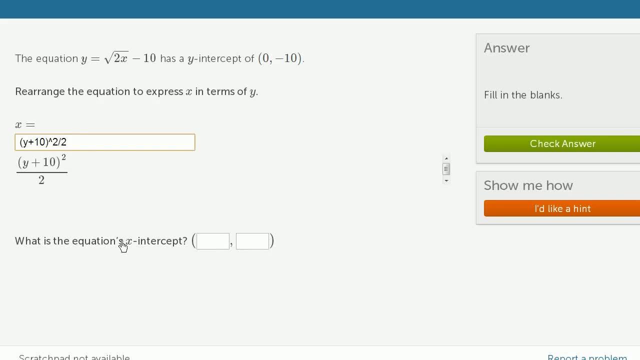 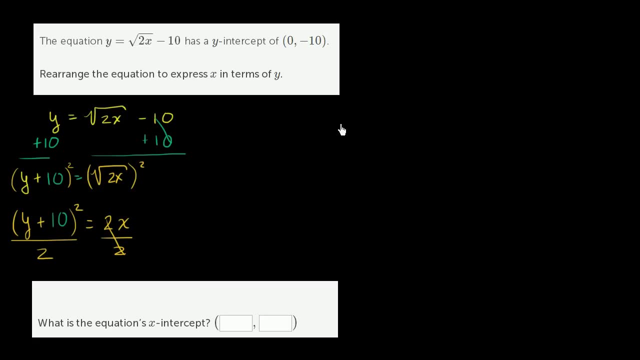 which is exactly what I wrote down on my scratch pad. And then they say: what is the equation's x-intercept? So let's just remind ourselves what's going on here. So this curve or this equation could describe a curve that looks something like this: 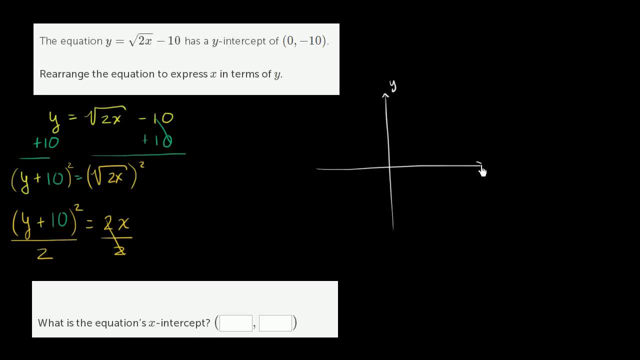 So this is my y-axis, This is my x-axis, And let's say the curve, It might look something like this, It might look something like that. So we already figured out its y-intercept. Its y-intercept is: where does it intersect the y-axis? 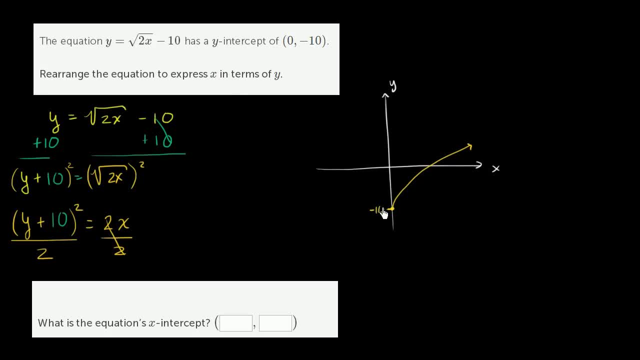 And we already figured out that's when x is equal to 0, y is equal to negative 10.. Now we want to figure out its x-intercept. So that's essentially, what x-value do we get to when y is equal to 0.. 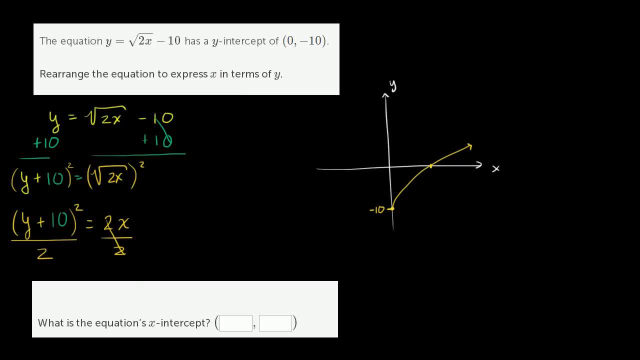 So what x-value do we get to when y is equal to 0?? Let me just clear these out, just so this doesn't get distracted by this right over here. Well, when y is equal to 0, x is going to be equal to 10 squared over 2.. 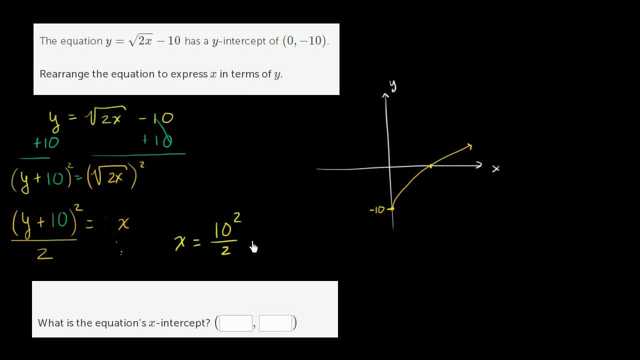 0 plus 10 is 10 squared 100 over 2, which is going to be equal to 50.. So we're at the point: x is 50 and y is 0.. So that's this right over here. The x-intercept is 50.. 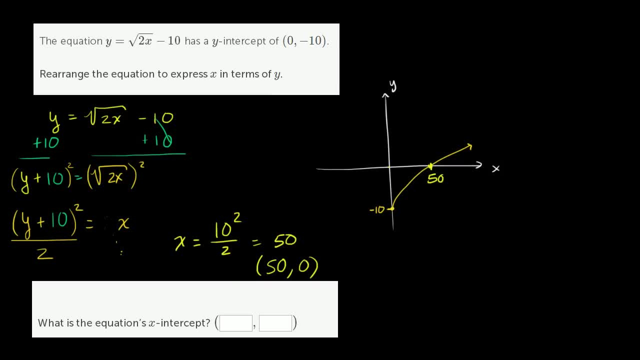 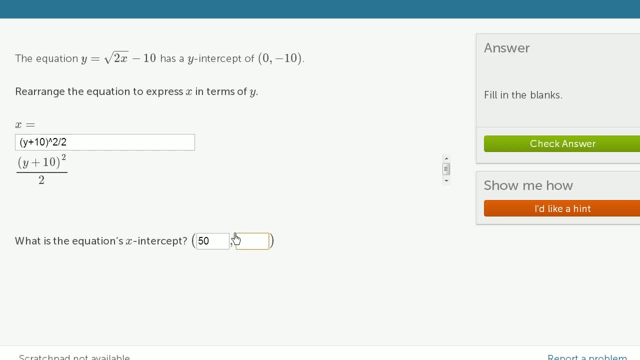 When x is 50,, we clearly see that y is equal to 0. So let's also put that in there. So what is the equation's x-intercept? So when x is 50, y is 0.. And we could check our answer and we got it right.